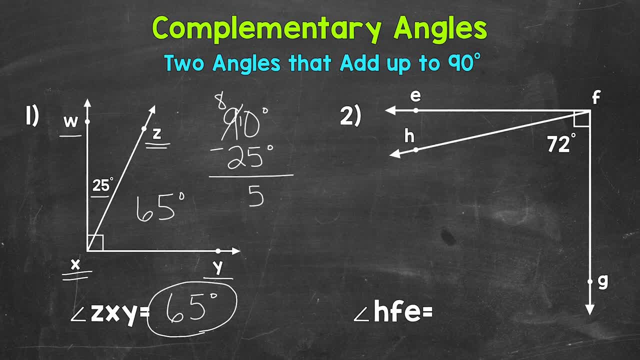 And we have 10 minus 5, which is 5.. And then 8 minus 2 is 6.. So we get 65 degrees that way as well. Again 90 degrees, because we know the two angles are going to add up to 90 degrees. 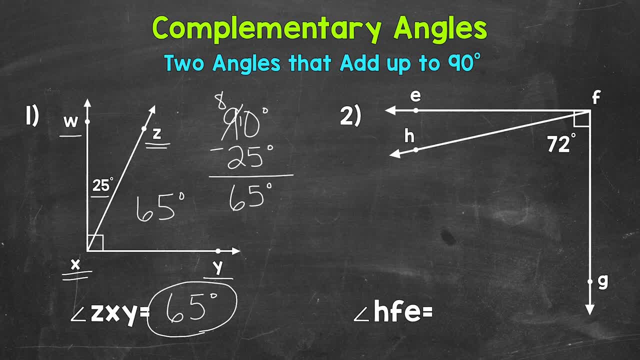 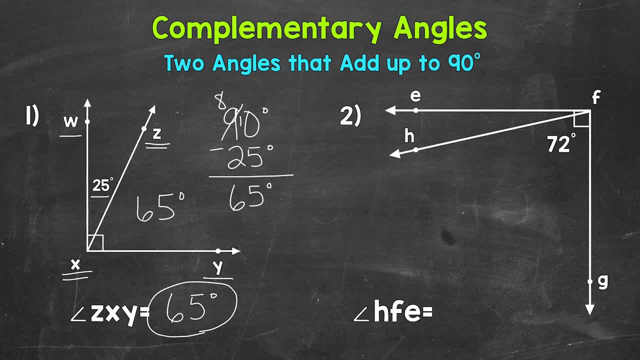 We can also subtract the given angle measure in order to get that missing angle measure. We can also check to see if our answer is correct by adding our two angles and then seeing if it equals 90 degrees. So let's double check here. We can do 65 degrees plus 25 degrees. 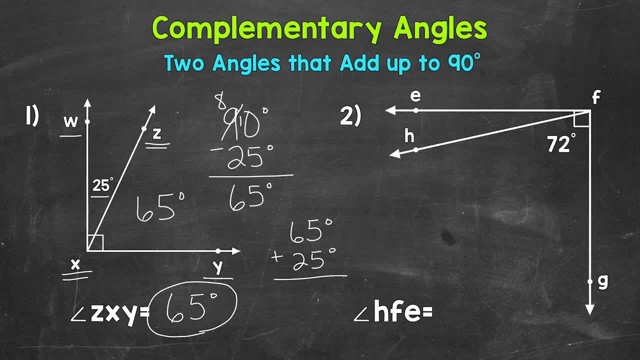 If that equals 90,, then we're good to go. 5 plus 5 is 10, so we have a 0 here, Carry. the 1.. 1 plus 6 is 7 plus 2 is 9.. So those two angles equal 90.. We have the correct answer there. The missing angle. 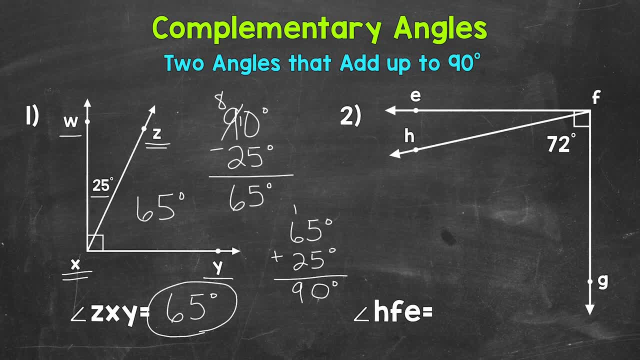 there is 65 degrees. Let's try another example here and move on to number 2, where we have a given angle measure of 72 degrees. So angle GFH equals 72 degrees. We need to figure out angle HFH, So let's do 90 degrees. We have complementary angles here, so we know they are going to equal. 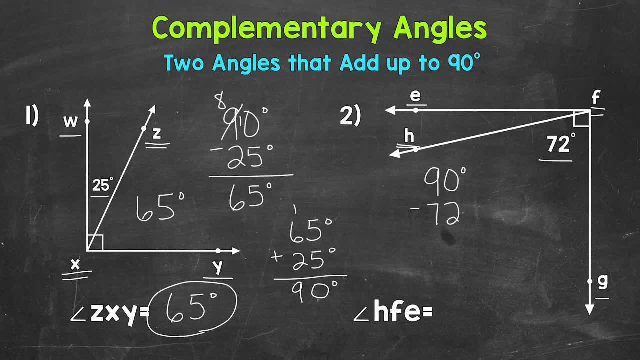 90, and we are going to subtract the given angle measure. Now again, if you can figure this out mentally, that's great, That works. But if not, that's fine too. We can always write out a subtraction problem to find that angle. So we have 0 minus 2.. Let's borrow. 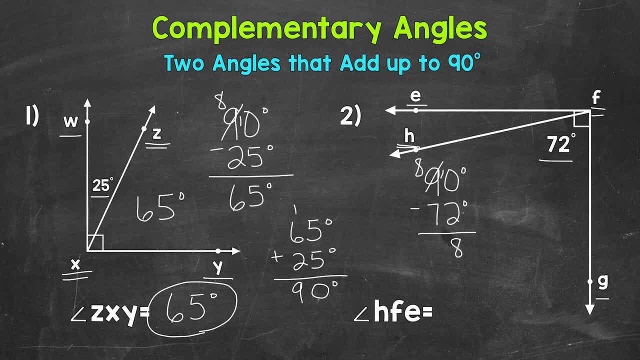 We have 10 minus 2, which is 8.. And then 8 minus 7,, 1.. So our missing angle, angle HFE- is going to be 18 degrees. Let's double check to make sure. So we'll do 72 degrees plus 18 degrees.